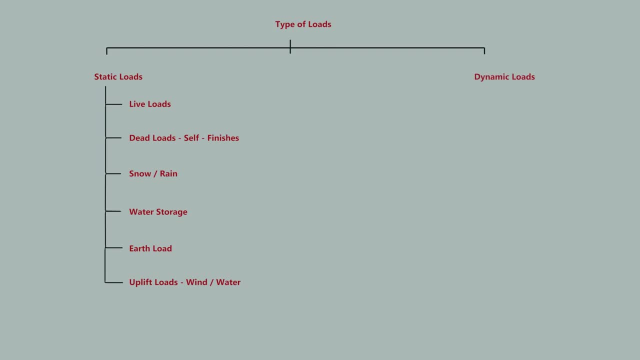 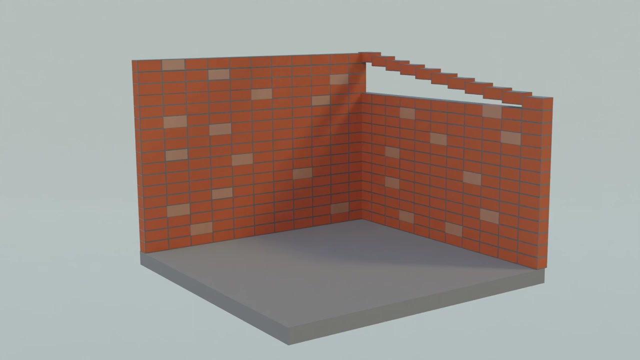 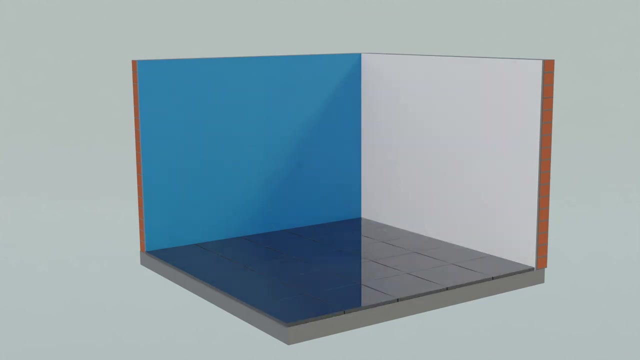 and uplift pressures. Dynamic loads, including earthquake, wind waves, blast load, traffic and earth loads. Loads that remain constant throughout structures, Structure life- are classified as dead loads, including brick, plaster, paint, fixed doors and windows, while life load depends on usage of space. Same space can be used as a bedroom. 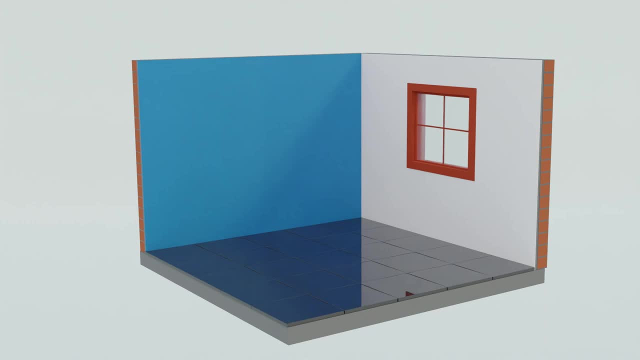 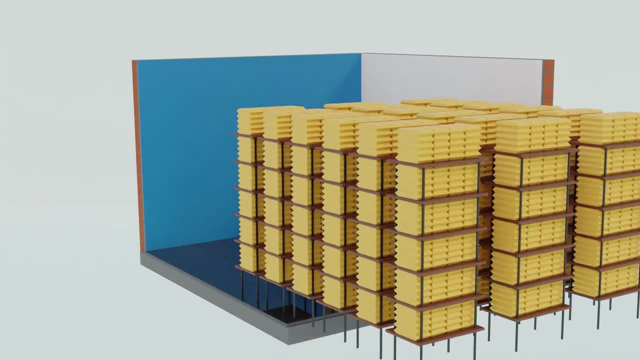 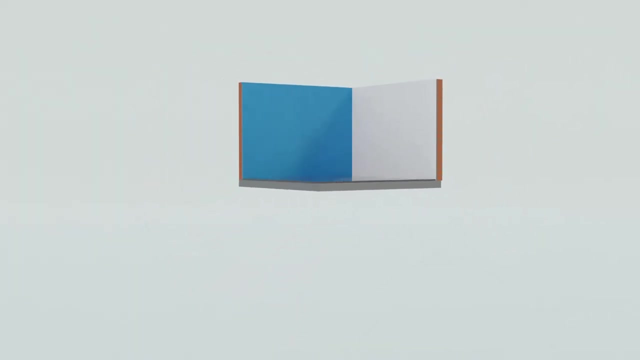 a classroom with chairs and several students, a dining with few people having dinner, a storage full of racks of wheat and containers. Water load can be caused by an overhead water tank or underground water tank, where load acts vertically on slab and horizontally on walls. 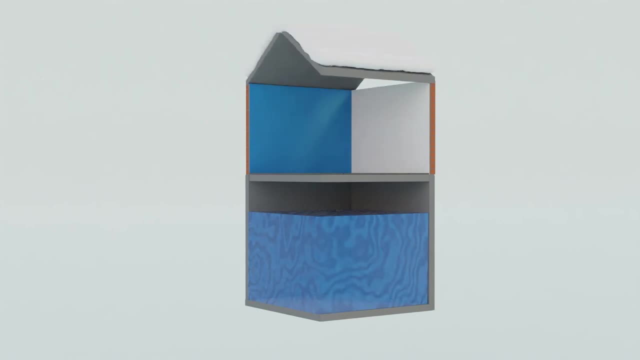 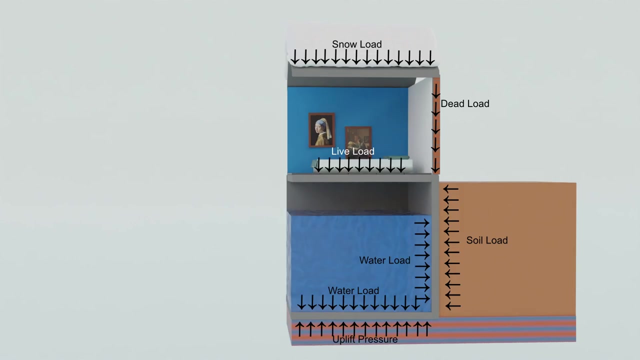 Rain and snow loads act on roof and can be countered by providing an inclined roof. Earth load is applied by soil on the walls of basement. Water present in soil can cause uplift on base of structures. Directions of load are shown here and building is designed to resist these forces safely. 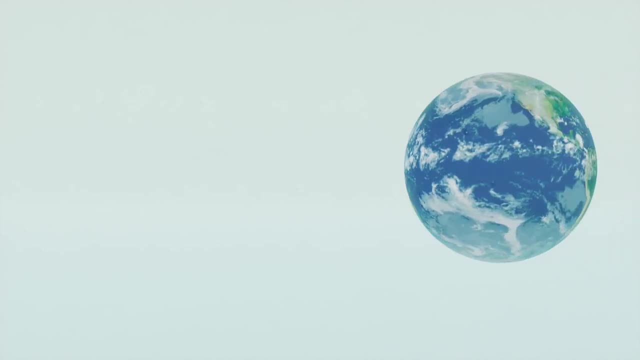 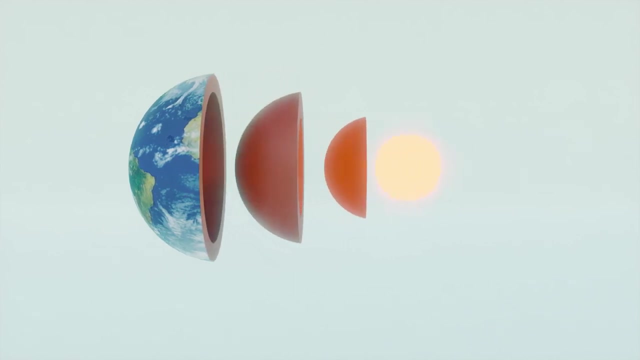 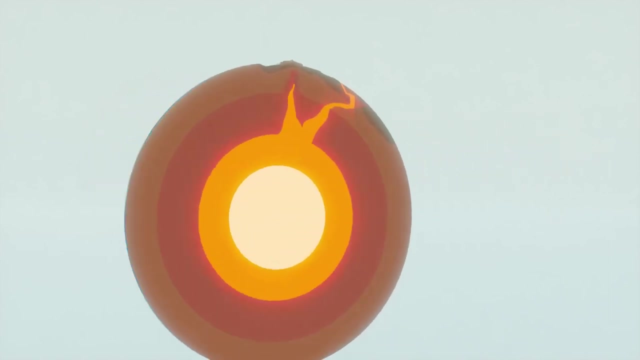 To understand an earthquake, we need to look into what the earth is made of. We live on the crust. Below the crust there is mantle. Below the mantle there is outer core and then inner hot core. They constantly push on one another. 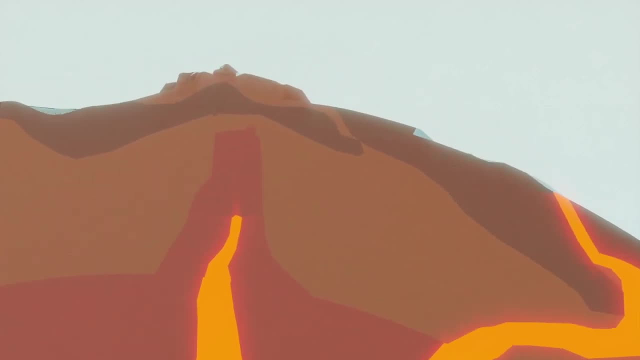 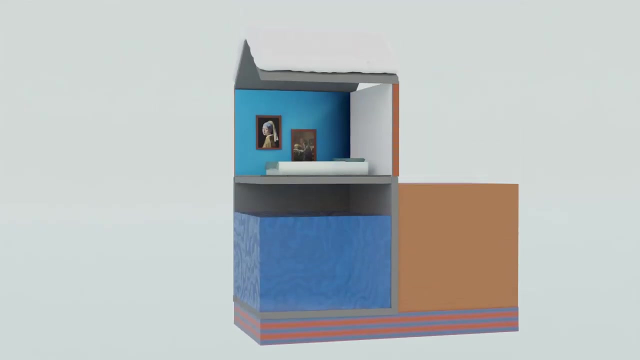 Either tectonic plates move and strike one another or magma tries to come out of the earth by pushing it and causing an earthquake. This phenomena results in changing of static loads to dynamic forces applied on structures. Soil and water start to apply forces on the wall. 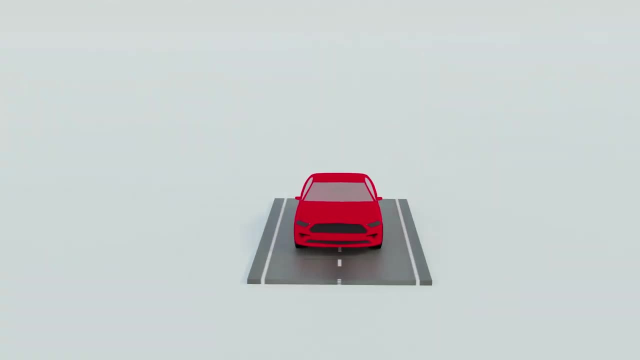 Other loads include the car on road, the weight, the force produced by brakes and the temperature load generated by the tires, The load of water and soil on the tunnel during construction and operation of the structure, Massive thrust produced by rocket propulsion and heat load produced by the fuel during combustion.